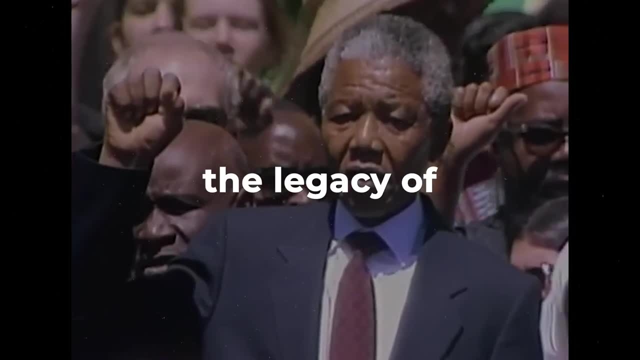 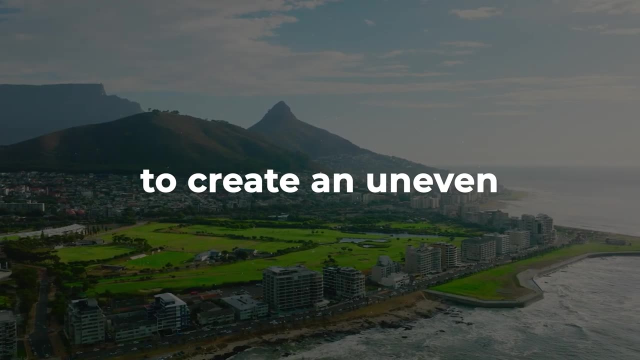 In 1994, thanks to the likes of Nelson Mandela, tax rate cuts, andytic inflation occurred, allowing people to be deprived of sizable jobs. A legacy of these discriminatory policies persists Despite the implementation of liberal policies. disparities continue to create an uneven playing. 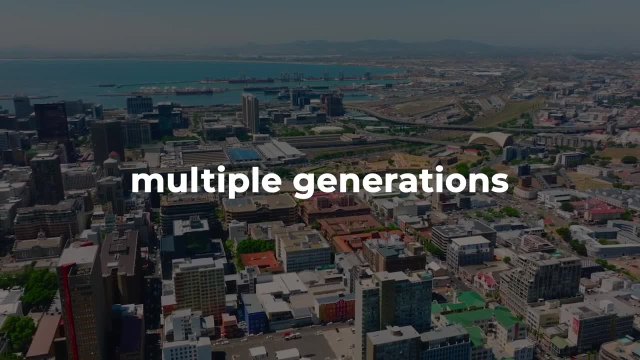 field. It has proven an impossible task to overcome multiple generations of extreme inequality in the space of a single generation. We're still dealing with an entire class of immigrants here with the hospital phones, So what we still have to do is push for the lockdown. but while putting a special name on the legal perfect to create equality, we're having to say the exact opposite in a tax but unbiased way. Much of everything that the Gini 있으 Humans can Doing, but we're also doing everything that the auto tech needs, and try making sure. 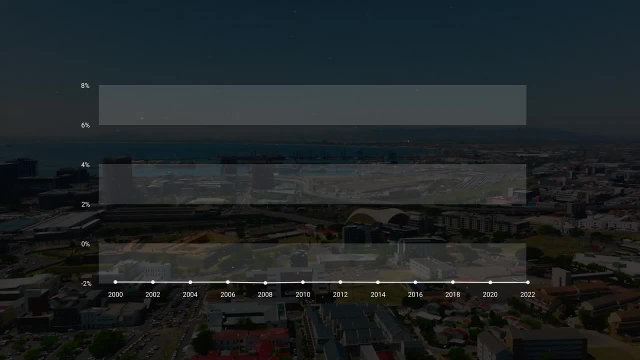 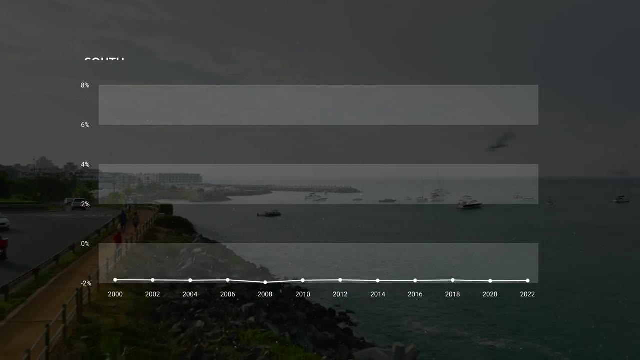 that we are providing important benefits based on what we really have. Another problem holding this fight back is the general lack of economic growth. This is the GDP growth chart since the turn of the century. When the economy is barely expanding, it becomes difficult to provide opportunities for the most disadvantaged, The rising unemployment and poverty. 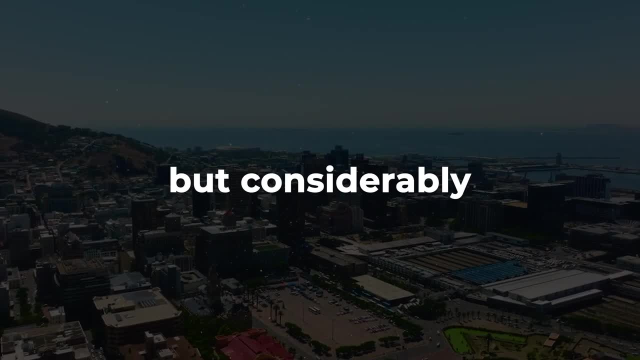 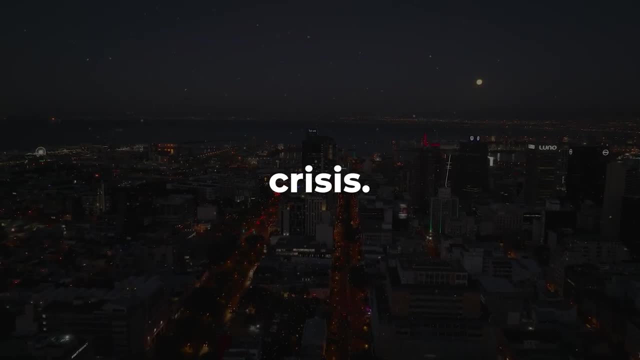 rates suggest that conditions have not just stagnated but considerably worsened in recent years. There are many reasons for this. One major hurdle is the ongoing energy crisis. Crippling power cuts, known as load shedding, are a daily reality for South Africans. These blackouts 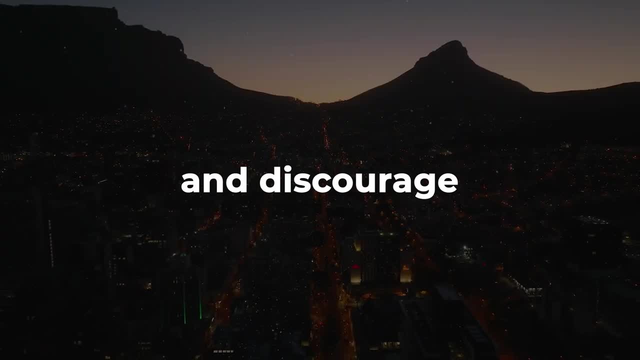 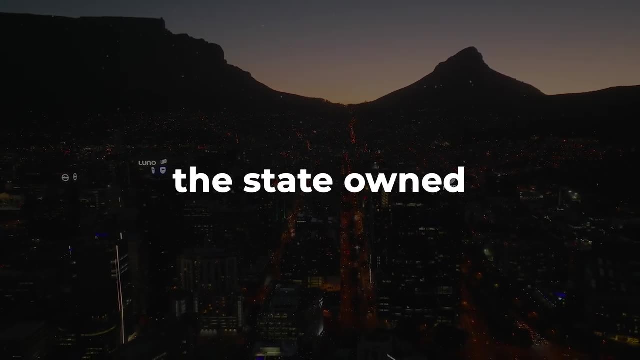 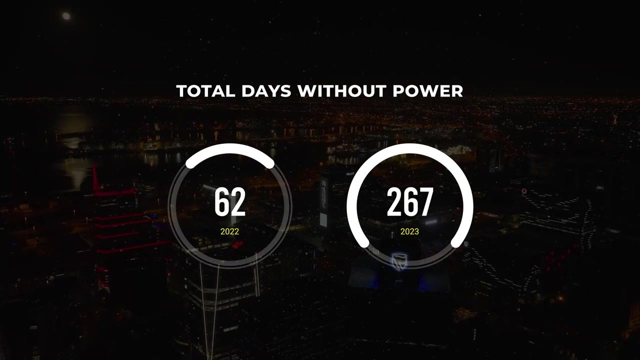 severely disrupt businesses, stifle productivity and discourage investment, preventing consistent growth. The root cause lies in the mismanagement and underfunding of ESCOM, the state-owned electricity provider. Last year, ESCOM cut power to households and companies for a record 280 days. 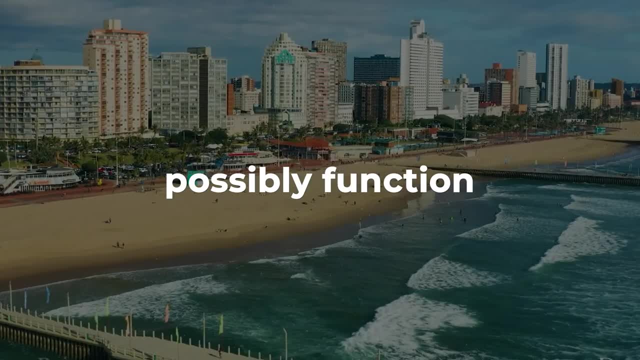 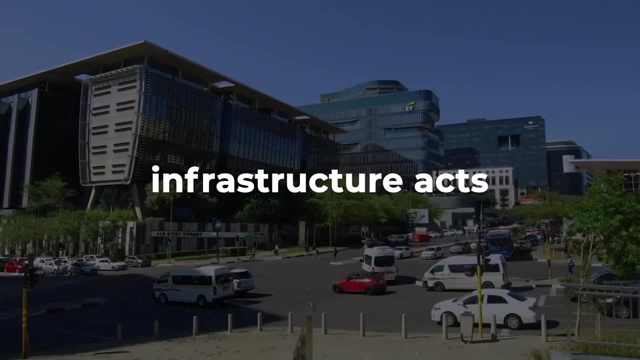 up from 65 days the year before. How can a country possibly function when, for up to 12 hours a day, households and businesses are left without any power? Crumbling infrastructure acts as yet another break on the economy. Roads, ports and other essential networks haven't received adequate maintenance and investment for 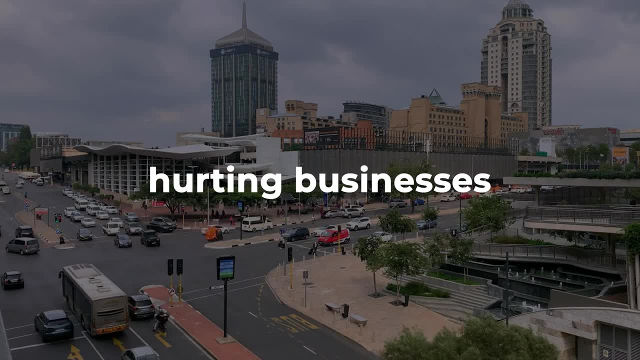 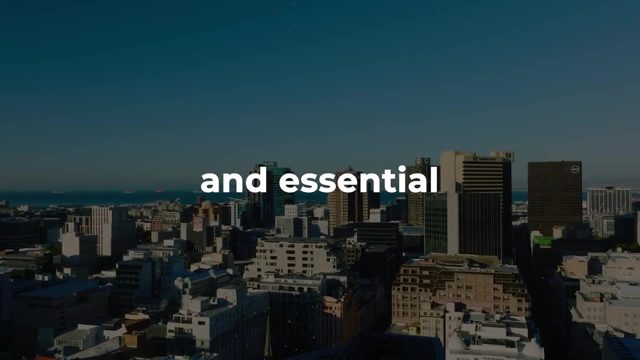 years. This makes the movement of goods more difficult and costlier, hurting businesses and, ultimately, ordinary consumers. Corruption has also played a role in this mess. Public funds meant for development and essential services have been siphoned off by certain officials and networks. This has starved the economy of vital resources, leading to an erosion in government trust. The political situation is currently very tense, with an election due this year. Extreme populist parties have become increasingly popular. They champion the death penalty and the mass deportation of immigrants, of whom they blame for the uncontrollable crime and youth.